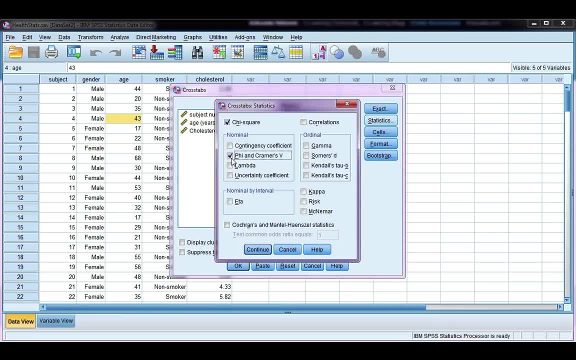 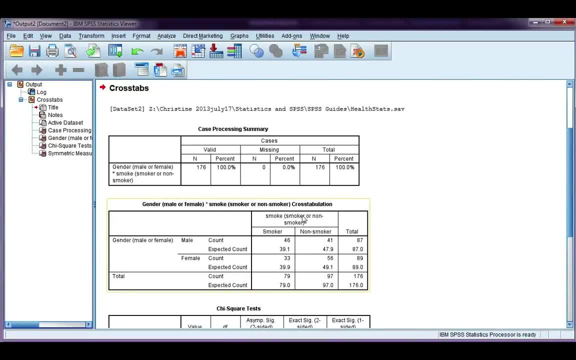 size of the table. So I'm going to go ahead and tick that box there, Go ahead and click continue and then click OK. OK, Let's look at our first table. This has our crosstabs and we have our observed count. 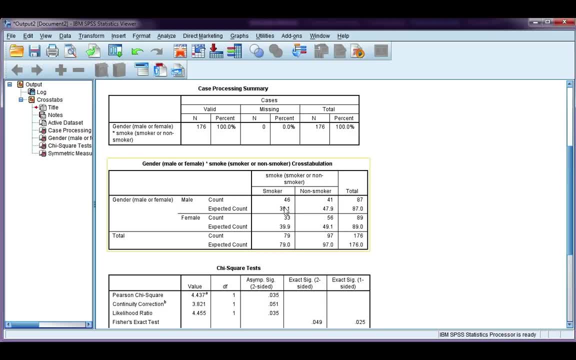 and we have our expected count. Now the expected count is what we would expect to observe if there was no association. So, for example, if gender had no relationship with smoking status, so gender was independent. So if gender had no relationship with smoking status, so gender was independent. So if gender 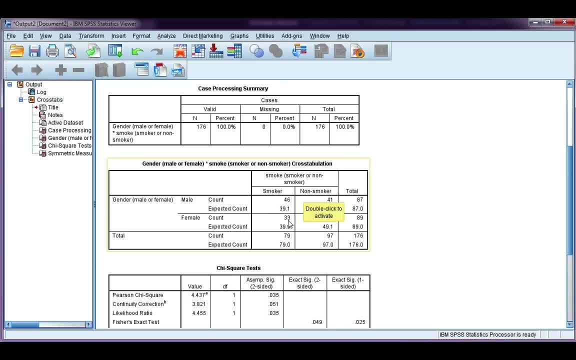 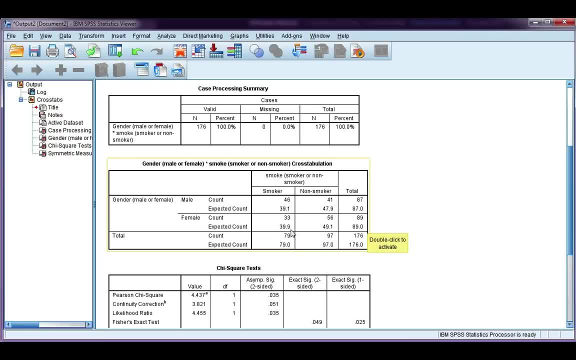 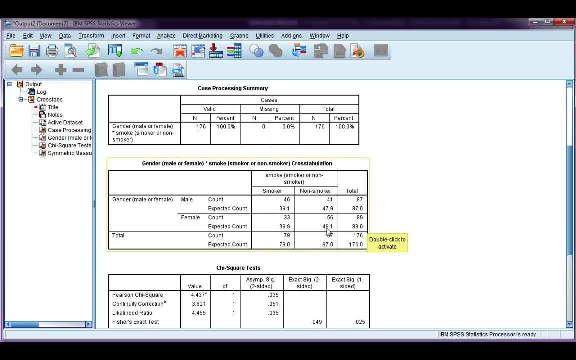 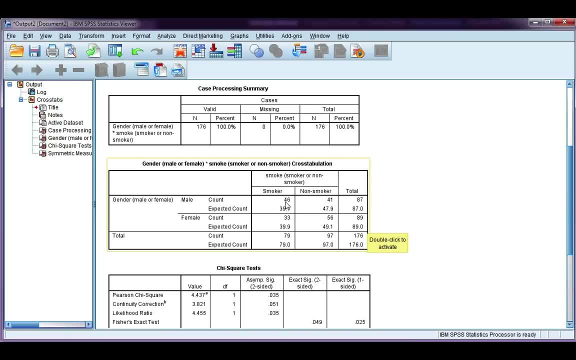 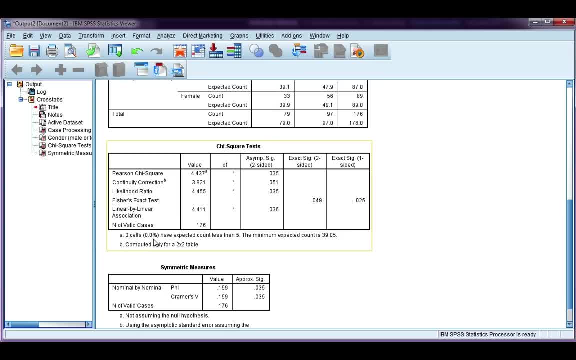 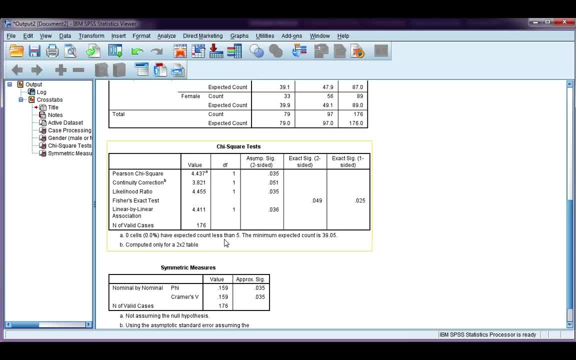 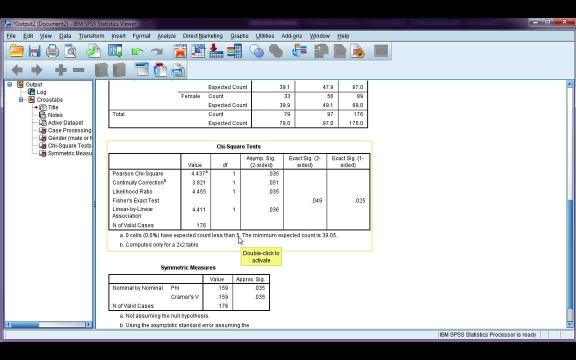 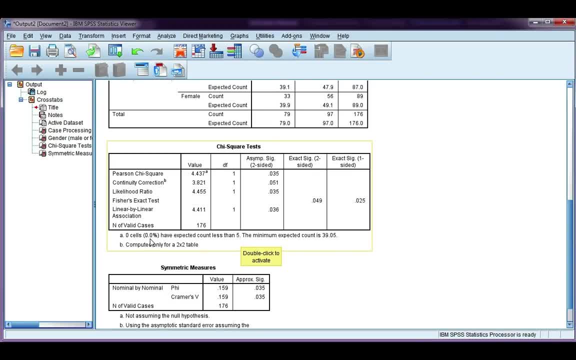 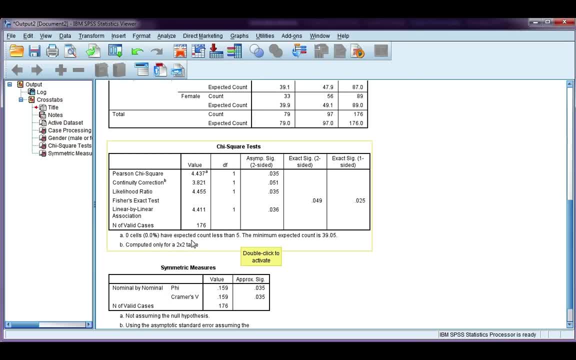 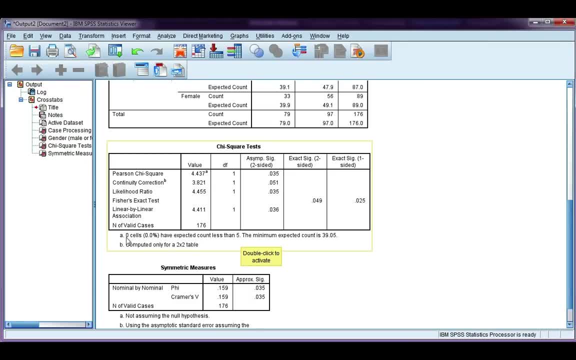 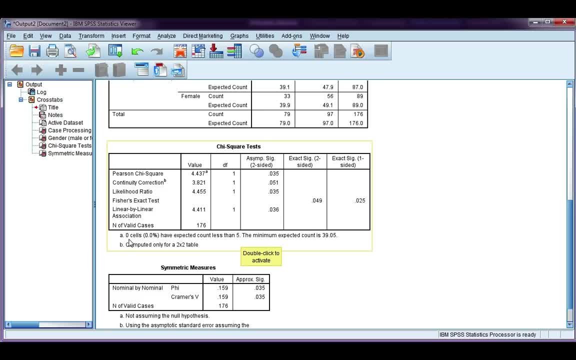 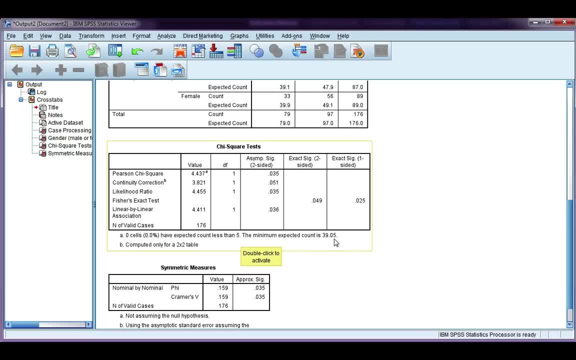 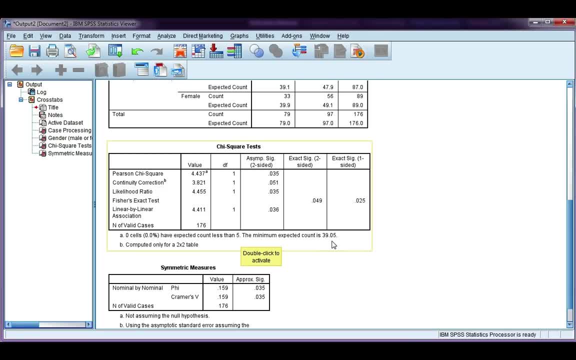 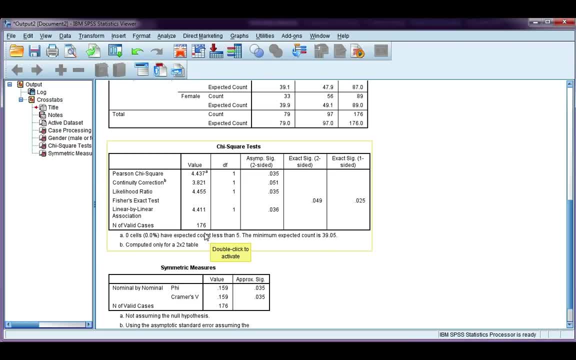 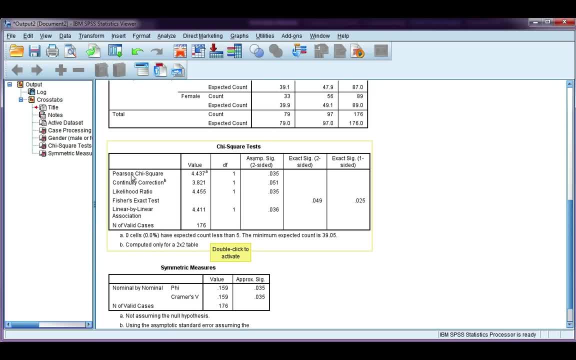 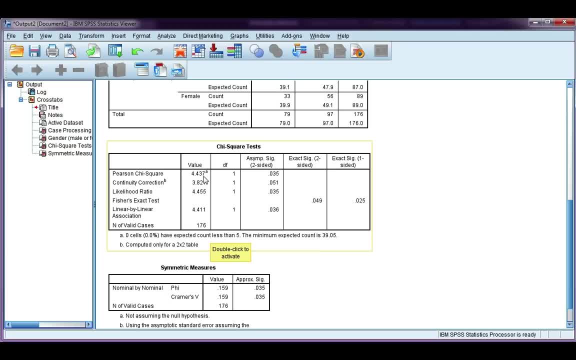 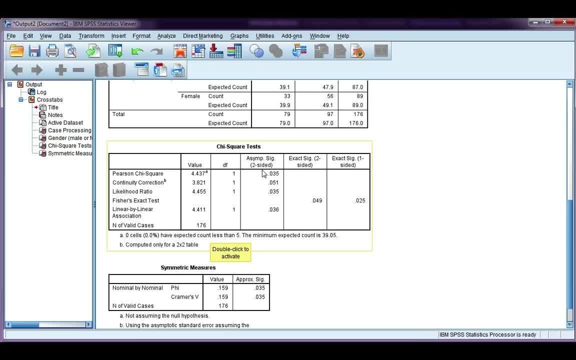 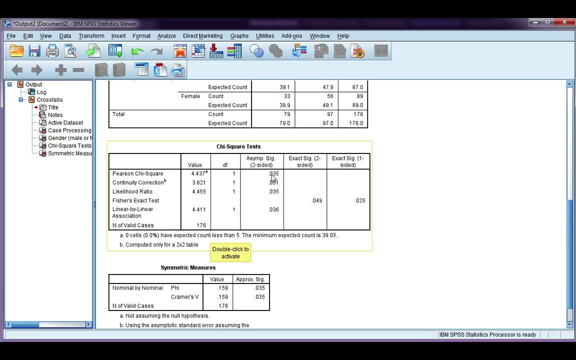 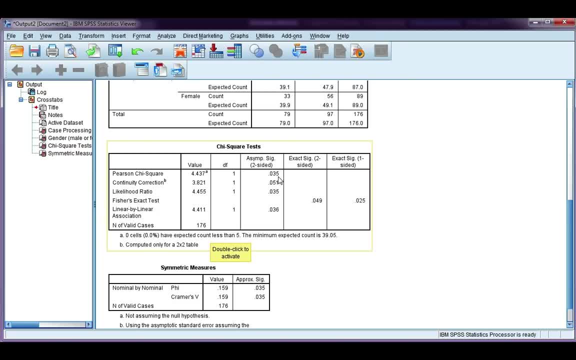 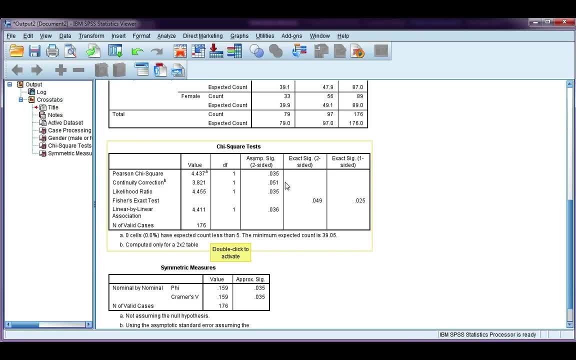 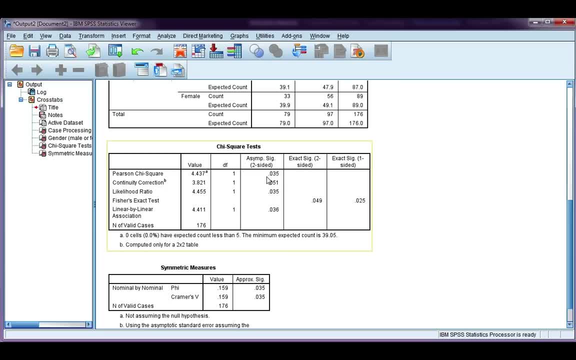 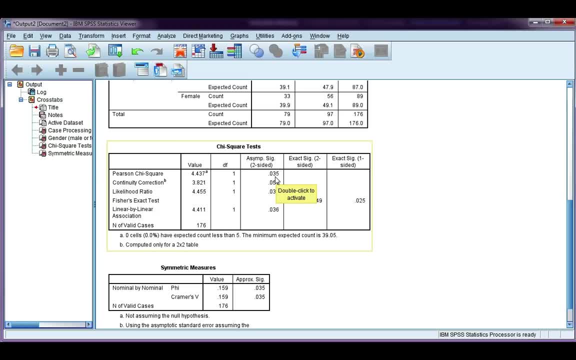 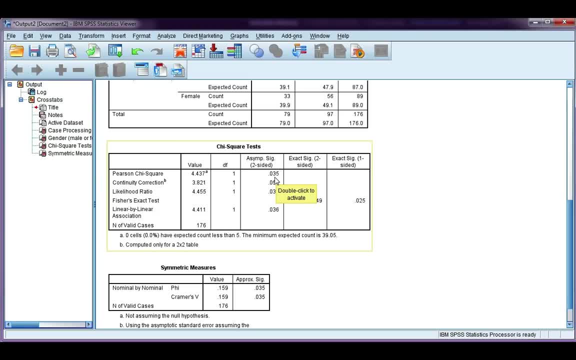 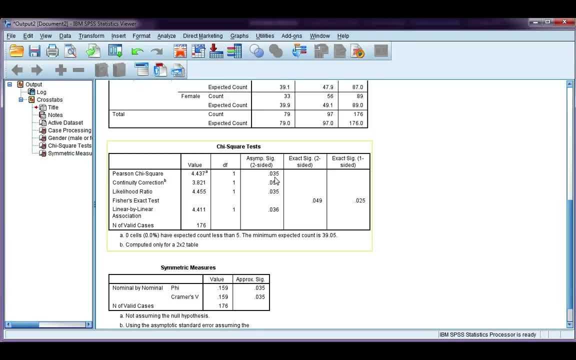 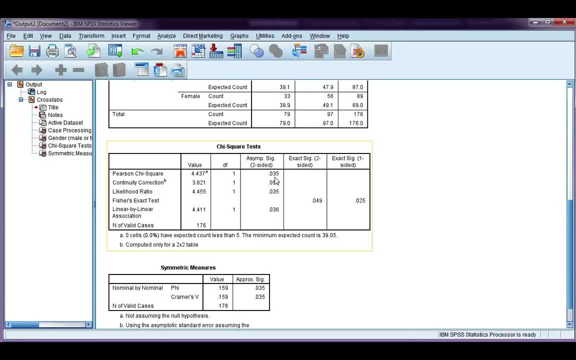 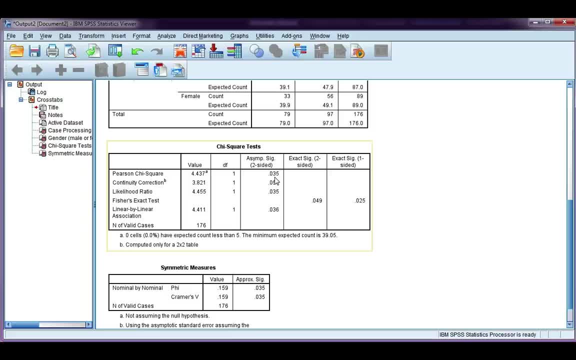 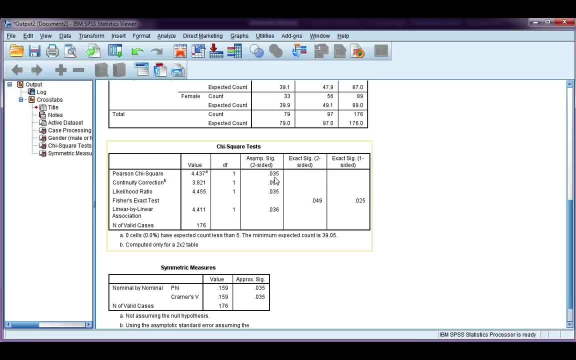 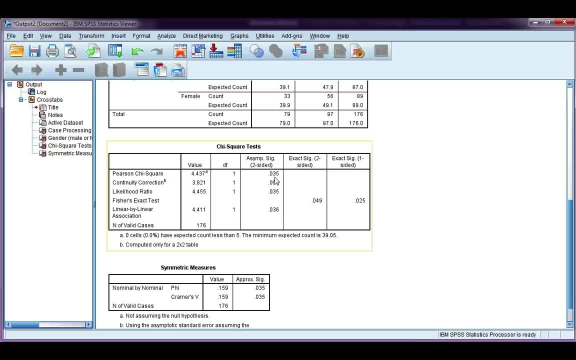 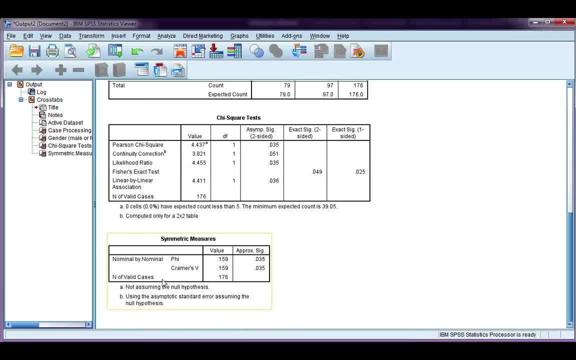 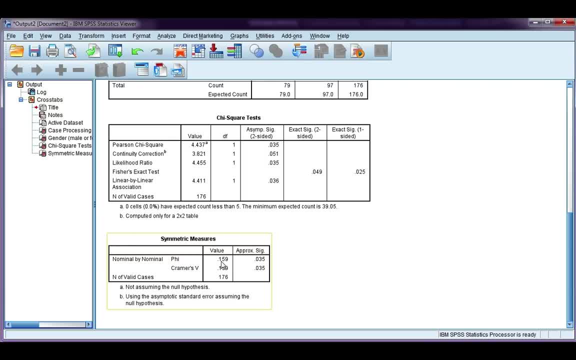 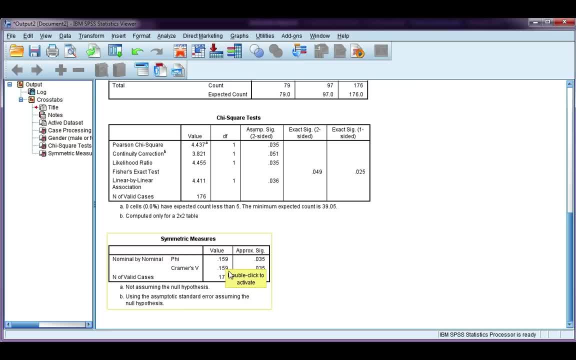 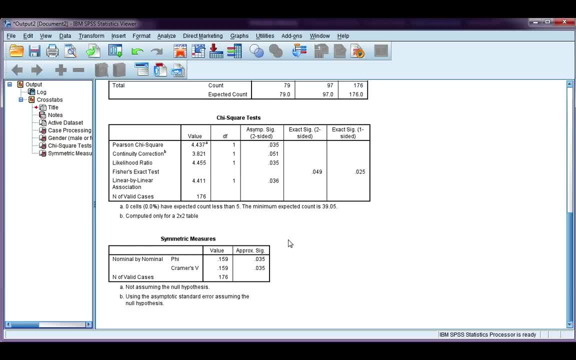 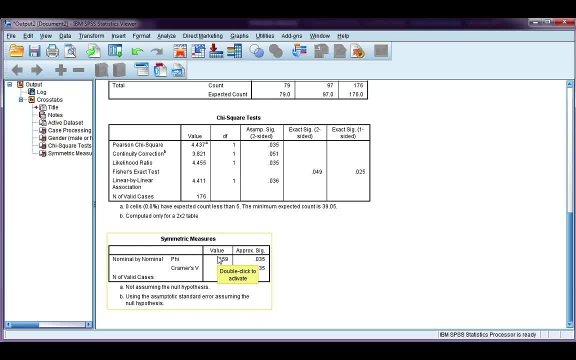 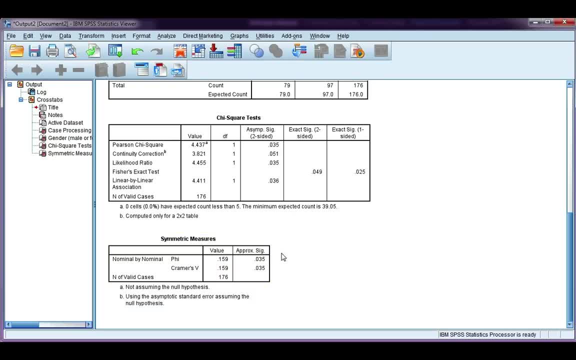 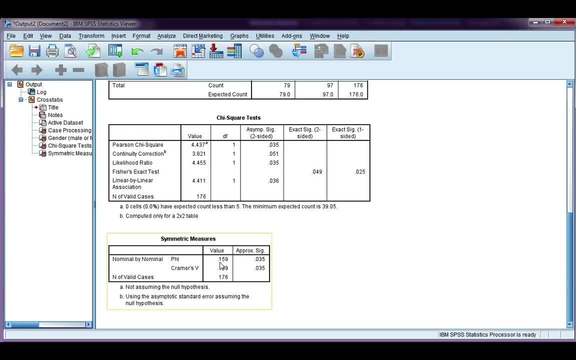 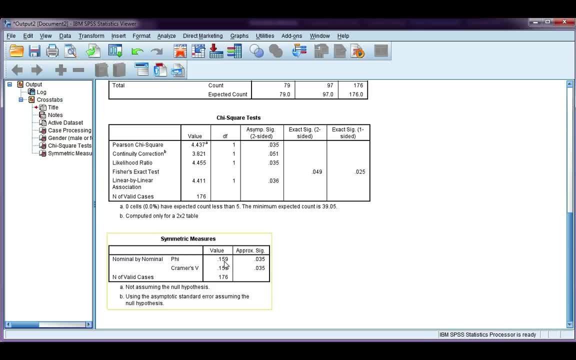 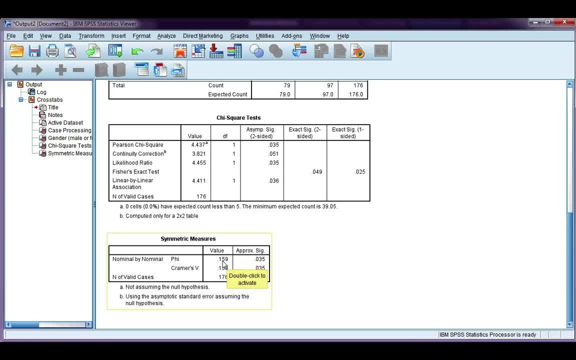 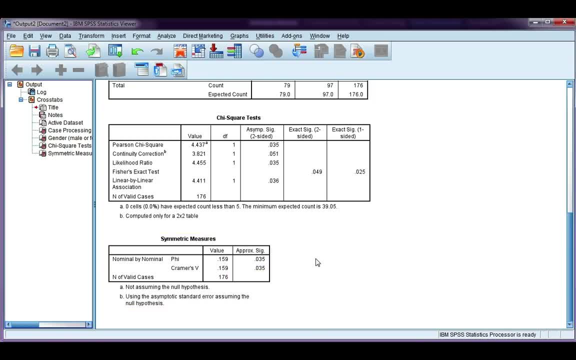 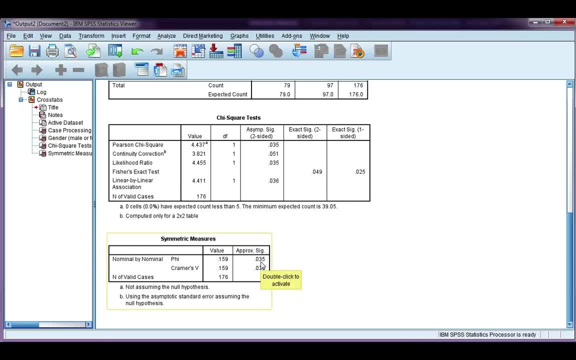